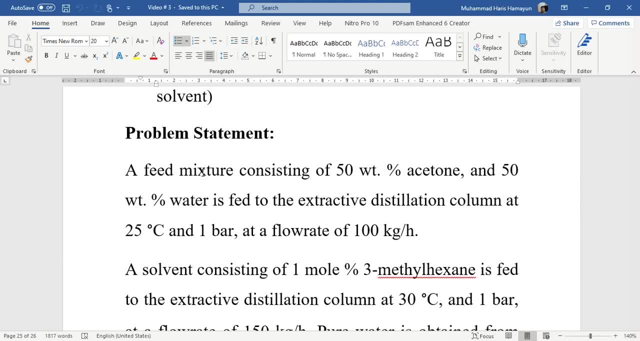 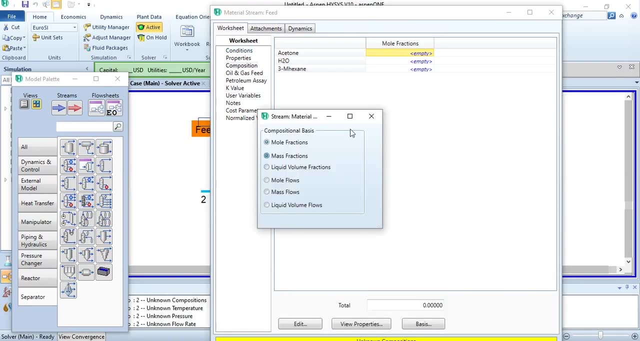 extractive distillation column at 25 degree centigrade and 1 bar, at a flow rate of 100 kg per hour. so we will first enter these values in stream number one, which we will label as feed. so in one feed: 25 degree centigrade, 1 bar, 100 kg per hour. mass fraction: 0.5 and 0.5 for both water. 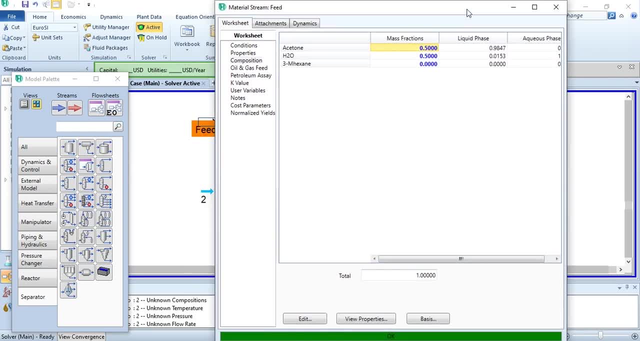 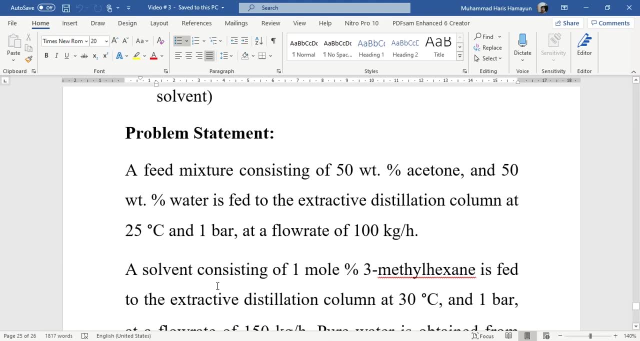 and acetone. it's converged as shown by the green bar. now, regarding the solvent, a solvent consisting of 5 m hexane and 1 bar at a flow rate of 100 kg per hour. so we will first enter these values. in of 1 mol percent, 3 methyl hexane is fed to the extractive distillation column at 30 degree. 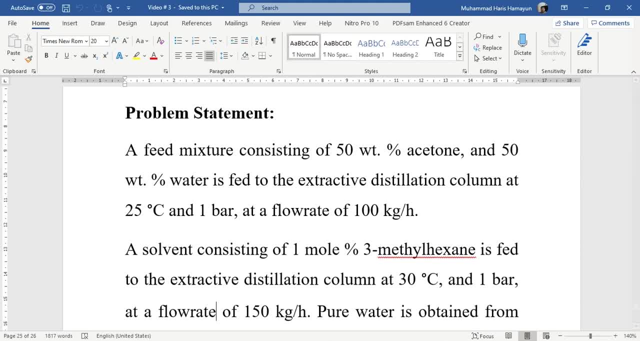 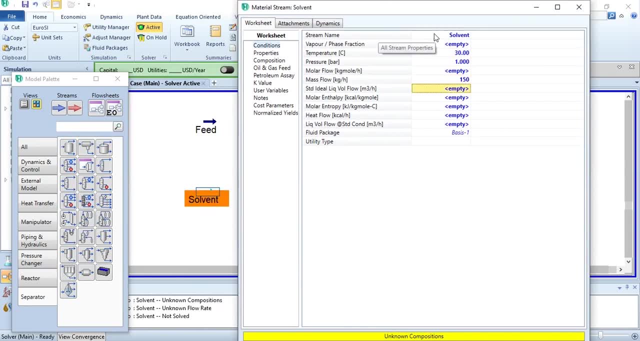 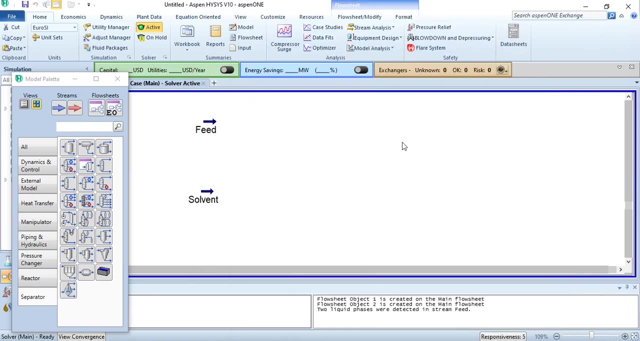 centigrade 1 bar, at a flow rate of 150 kg per hour. So we will click on 2 and we will label it as solvent stream: 30 degree centigrade 1 bar, 150 kg per hour. mole composition as 1 for 3 methyl hexane, and this has converged as well. Now we will have to add an extractive. 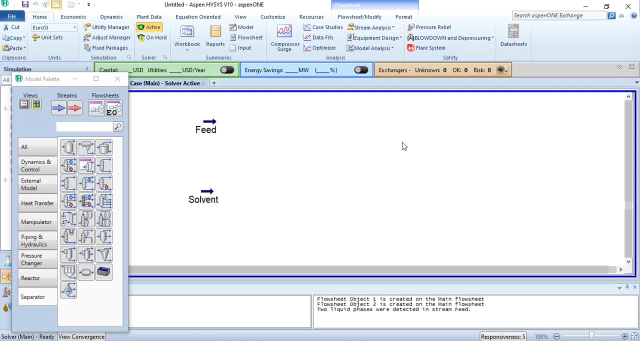 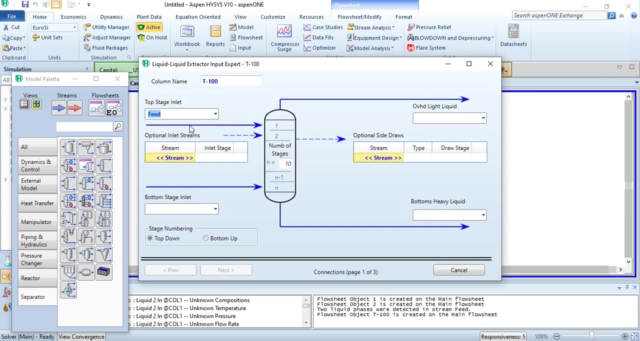 distillation column in which this feed and solvent will be fed and which is placed over here as liquid liquid extractor. So we will click it and we will place over here and first task, as you know, is to do the connections: feed- top stage inlet, bottom stage inlet solvent. we will label it. 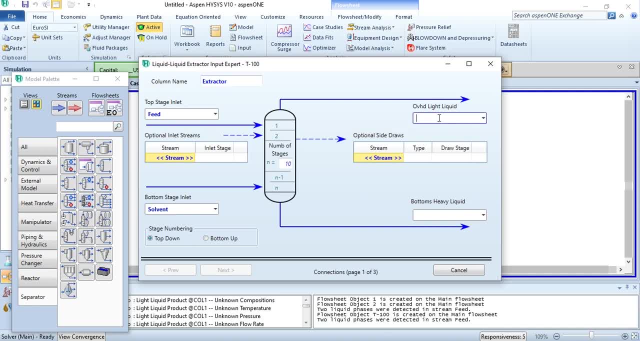 as extractor and overhead light liquid. we will label it as top product and bottom. obviously it's water. As we have discussed in our lecture number 13, that water will be obtained from the bottom of this column and this will be a pure water. Now we have to check: what is the information given to us? 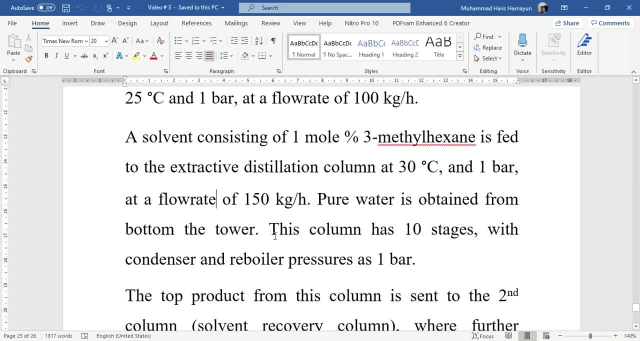 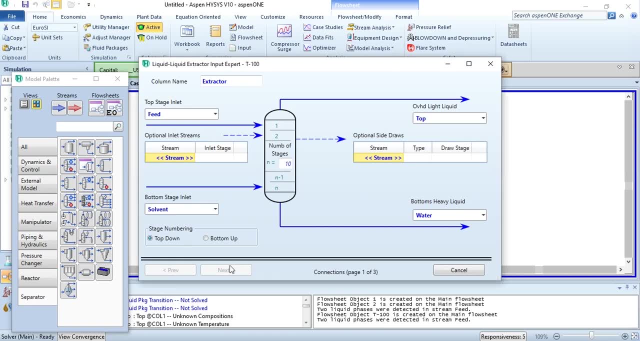 about the number of stages. Pure water is obtained from the tower. this column has 10 stages, with condenser and reboiler pressures as 1 bar. So the number of stages are 10. click next in condenser, which is the top stage- 1 bar. bottom stage- 1 bar. click next and obviously it's top stage and bottom. 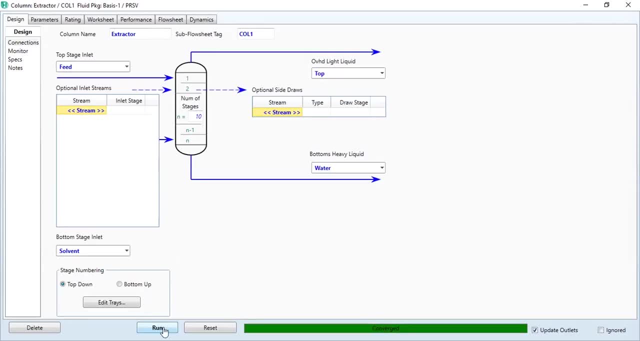 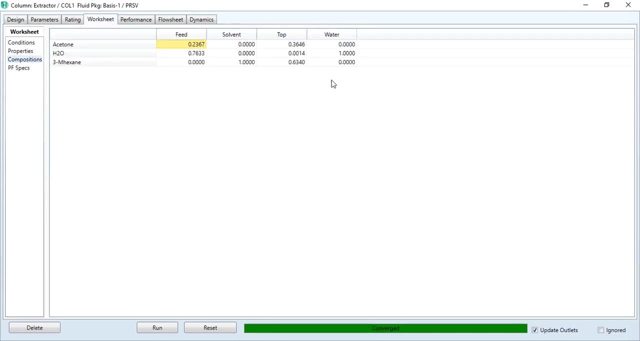 stage Pressures. so simply click, run after entering the values and you see this has converged successfully. So, going to worksheet and in composition, as you see, the water, it's mole fraction, is 1.. It means that this stream is purely water stream and the remaining stream, which contains mainly 3-methylhexane. 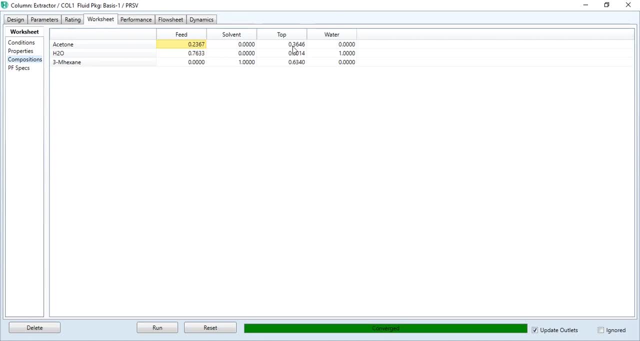 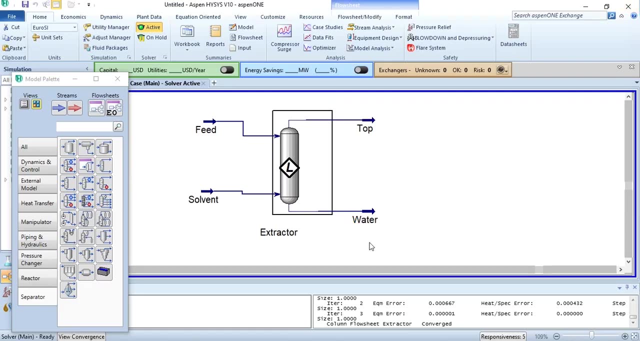 because it's solvent stream, acetone, which is separated from this feed stream, and very small quantity of water. So after computing this, we know that pure water is obtained from this extractor. Now this top, which is the mixture of acetone and 3-methylhexane, will be taken to the next column, which is the solvent. 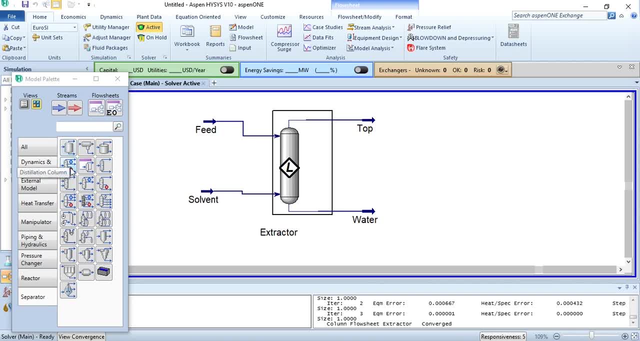 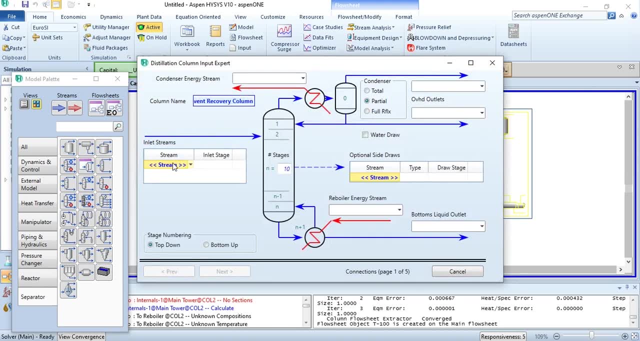 recovery column and this column will be the same column as that of distillation column. Now clicking on it and first we will label it as solvent recovery column, and inlet will be top and we will do the connections Q condenser, Q- reboiler, bottom is obviously the solvent recovery column and 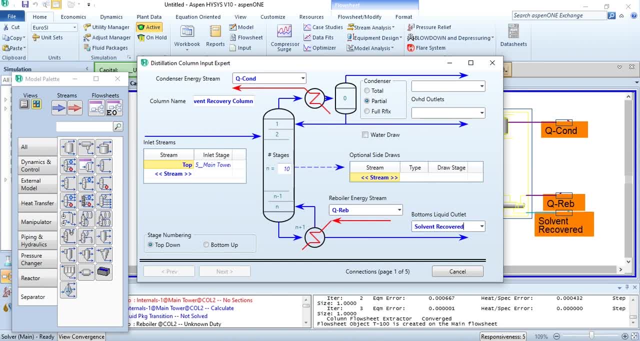 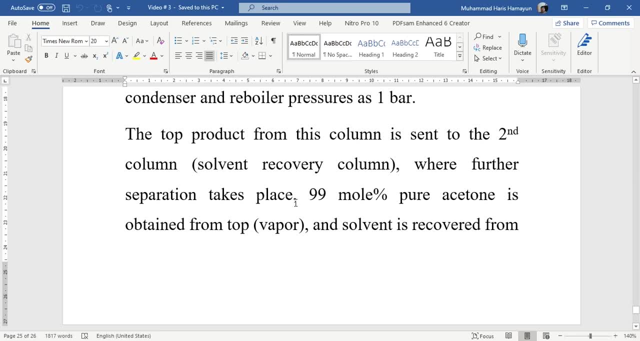 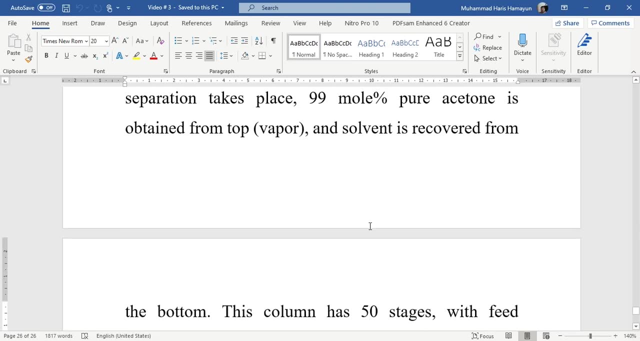 solvent recovered and for top. we have to go back to the problem statement. The top product from this column is sent to the second column, which is the solvent recovery column, where further separation takes place. 99% pure acetone is obtained from top which is in vapor state, and solvent is recovered from the. 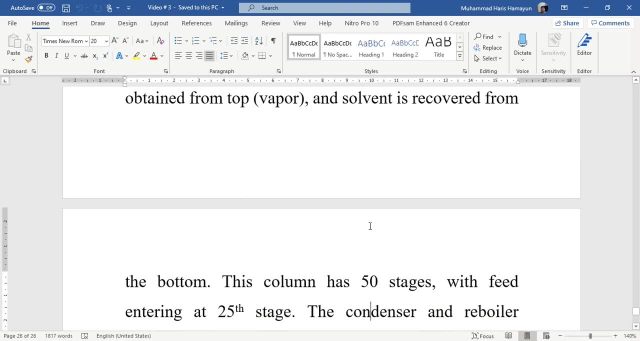 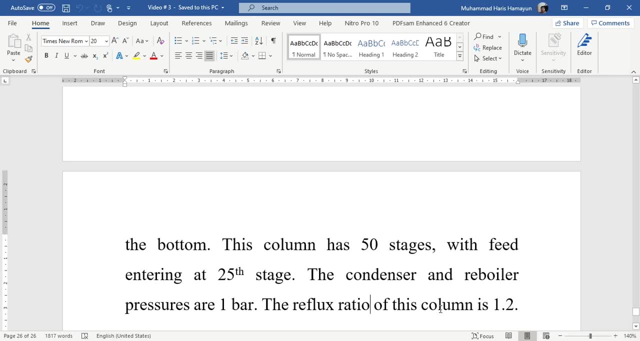 bottom. This column has 50 stages, with feed entering at 25th stage. The condenser and re-boiler pressures are 1 bar and the reflux ratio of this column is 1.2.. We have simulated this column several times so we know that we have. 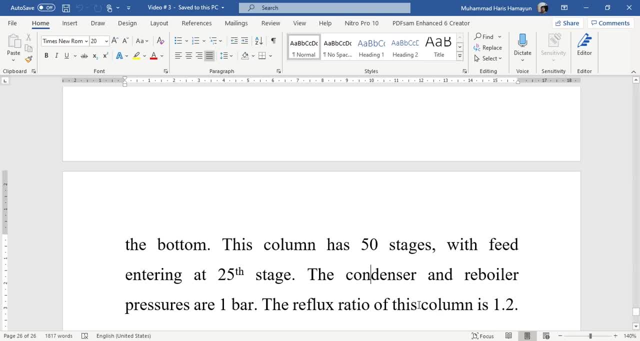 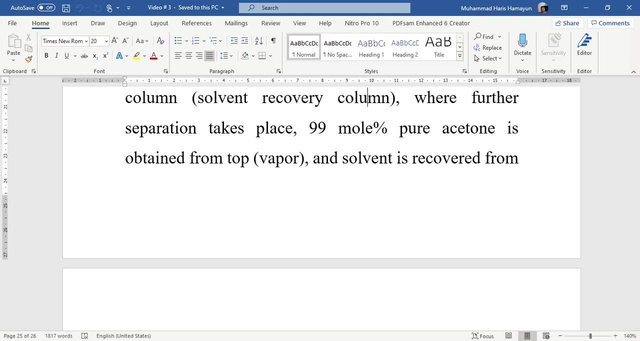 two design parameters. Number one is the reflux ratio of this column and number two is the 99% pure acetone, the purity of acetone in the top. So going back to aspen hyacinth, this column has 50 stages, with 25th stage as feed stage. 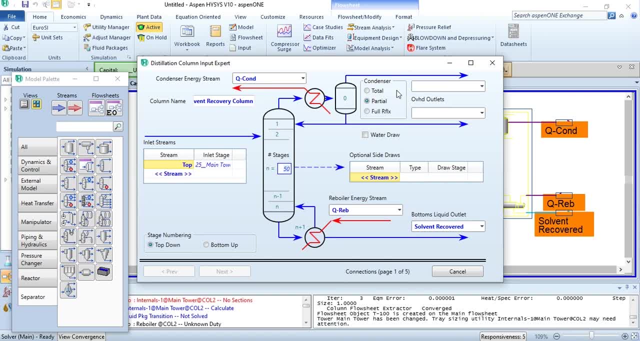 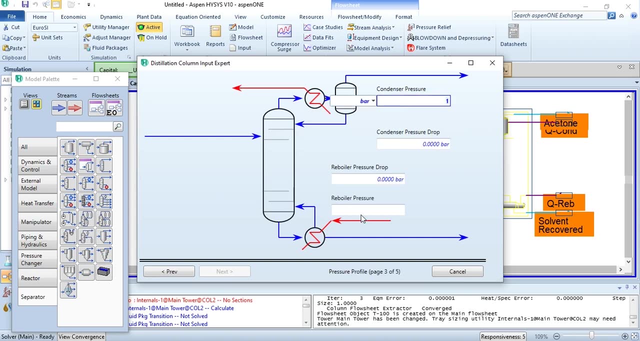 Now it's saying that the top product should be in vapor form. So we cannot select total, we cannot select partial. we will select full reflux and we will label it as acetone. After doing it, click Next and then regular hyacinth. re-boiler: condenser pressure: 1 bar. re-boiler pressure: 1 bar. again click. 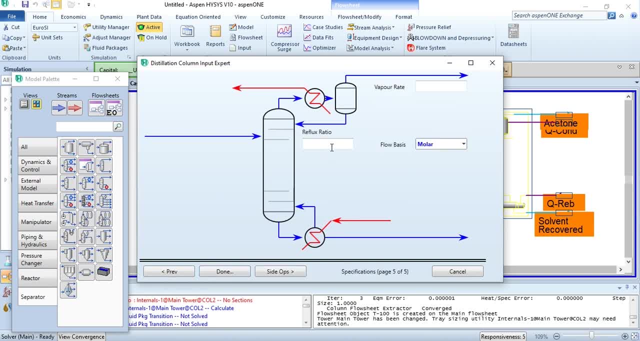 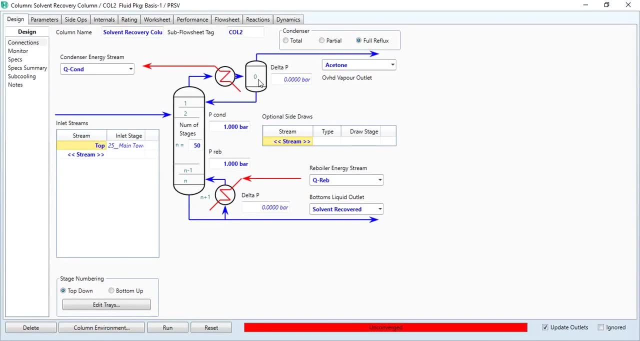 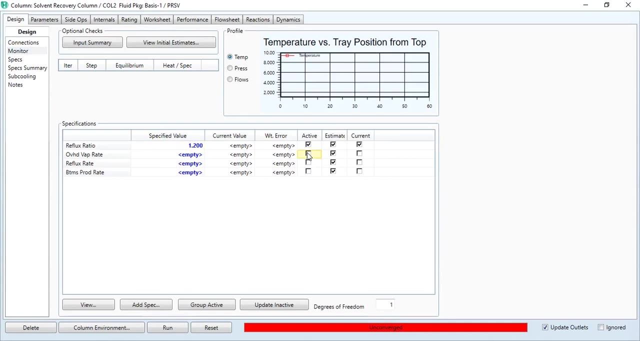 Next, No optional estimates given. click Next. and we have been given that reflux ratio is 1.2.. So, after entering this value, click Done. and obviously the degree of freedom is 1 because we haven't given one parameter yet. We will uncheck it and, as you see, degree of freedom has. 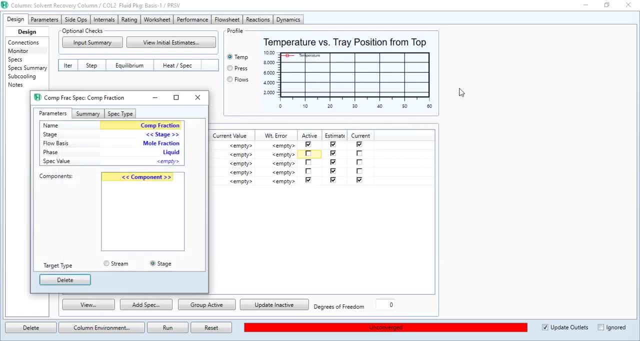 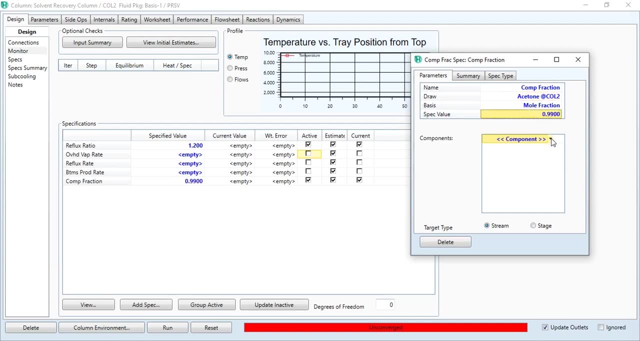 become 1.. So we will go to add spec and column component fraction In stream. we will select acetone, which is the top, whose mole fraction is 0.99 of acetone, Once after entering these two values, which is the reflux ratio and component. 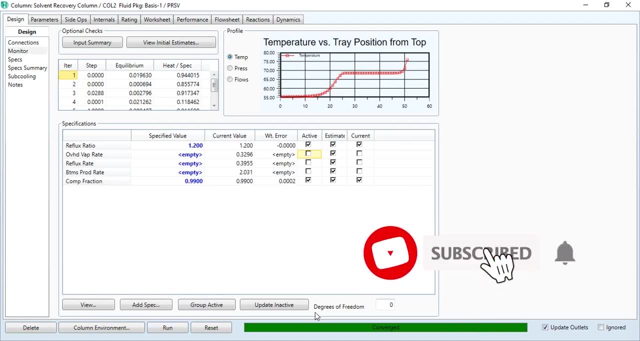 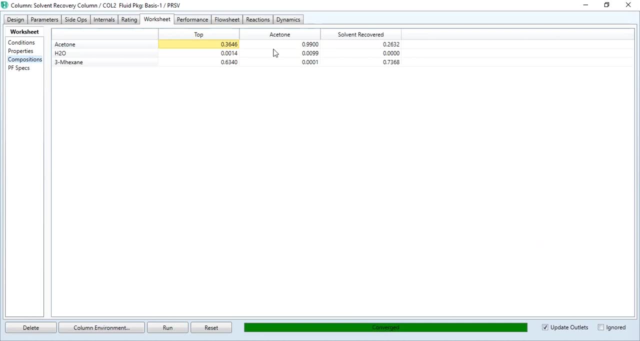 fraction, click Run and this column has converged successfully. Now going to worksheet: in composition, as you see, in the acetone stream, the acetone present is 99% pure. It means that acetone is 99% pure. This means that acetone is 99% pure. 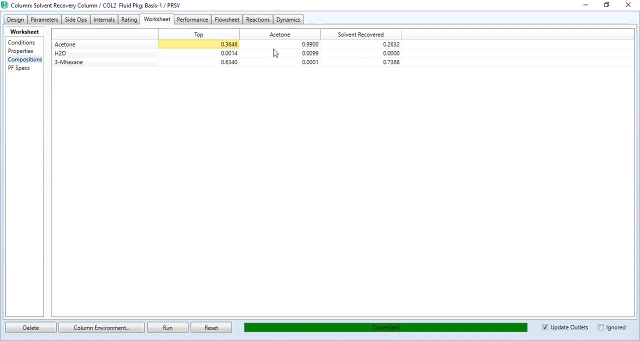 We have achieved our required target and in recovered solvent it's 73.68% solvent while 26.32% acetone. as depicted in the normal process, that 100% solvent is obviously recovered, but it contains some acetone as well. So our 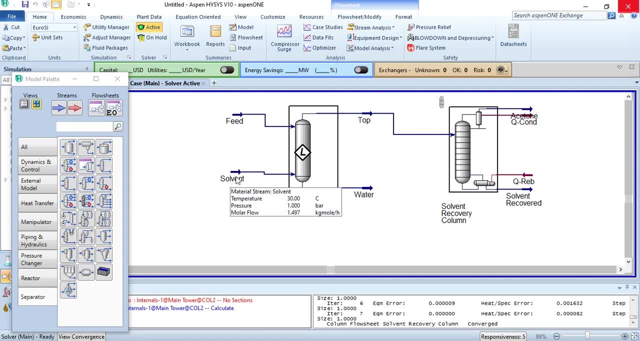 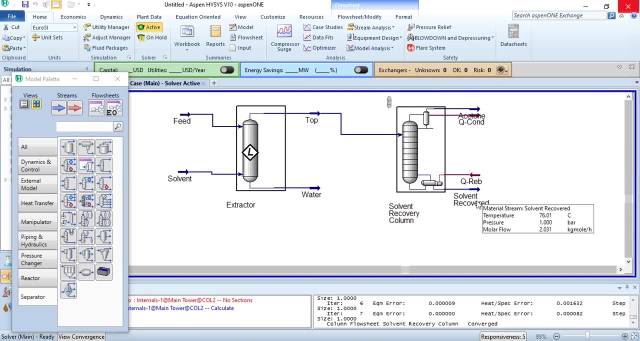 next task is to recycle back this solvent so that it can be reutilized. However, our first task is to cool down the solvent because currently the solvent is at 76.01 degree centigrade. So what we will do? we will select cooler. 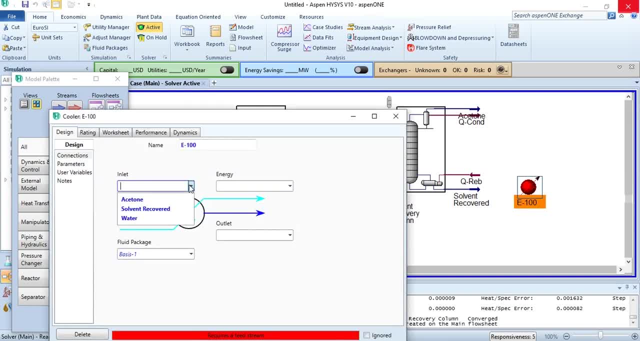 and we will cool down its temperature to 30 degree centigrade. solvent, recovered, Solvent 2. I will label it as Q cool and I will label it as cooler, and it's 30 degree centigrade and 1 bar. Now it's ready to be recycled. However, in our 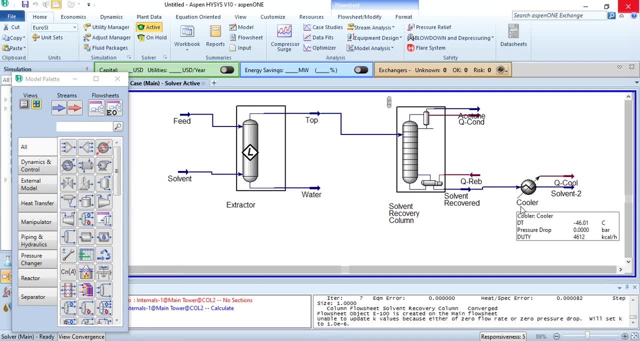 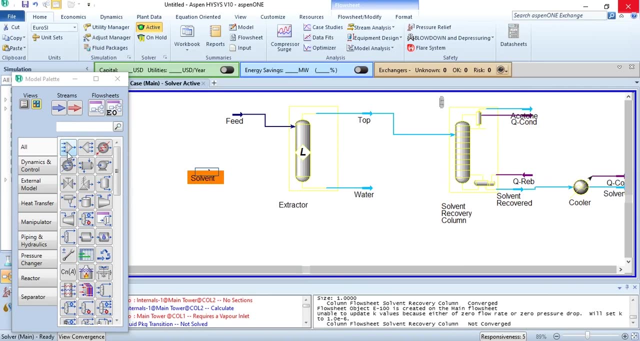 industrial processes, as you know that there is always a supply of fresh stream along with the recycle stream, So we have to also show it over here as well. So what I will do- simply remove the connections of solvent from here- and what I will do- I will use a mixer over. 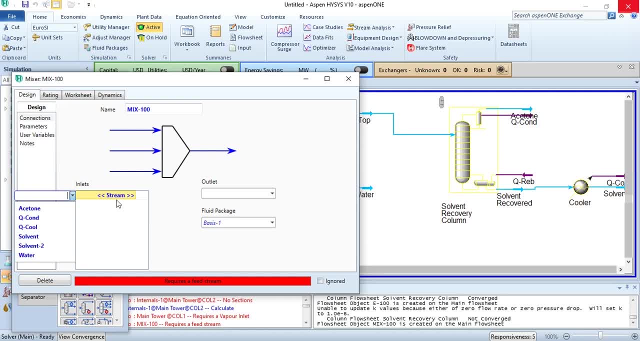 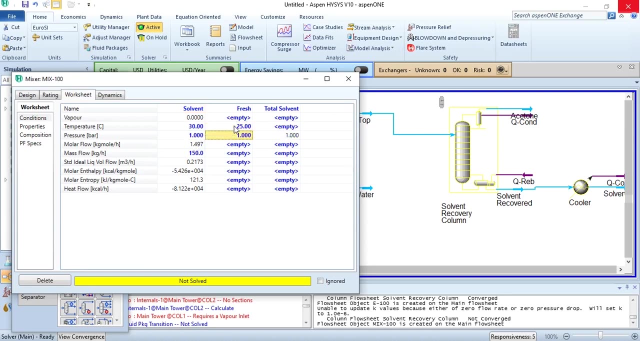 here and in this mixer I will add solvent and the fresh stream, which is the fresh solvent, and I will label it as the total solvent, which is a mixture of the solvent and the fresh stream. we have defined the solvent and the fresh stream. the fresh stream is 25 degree centigrade, 1 bar, and i will currently 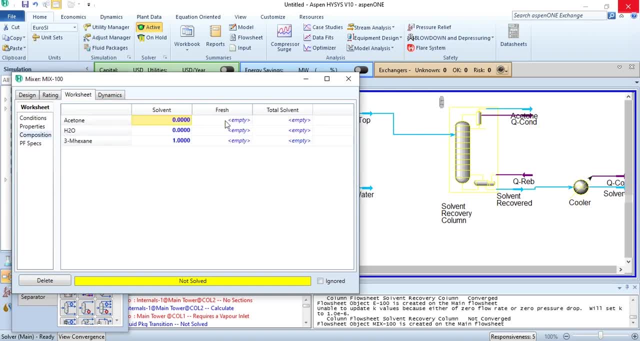 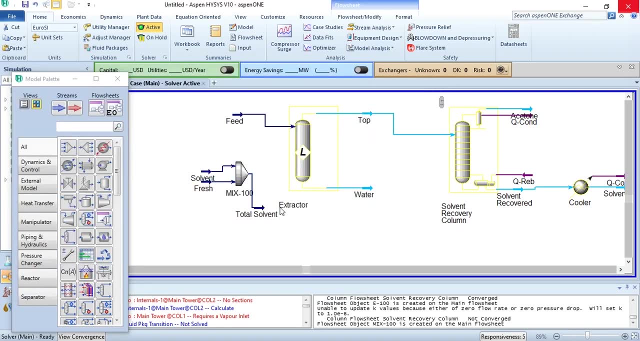 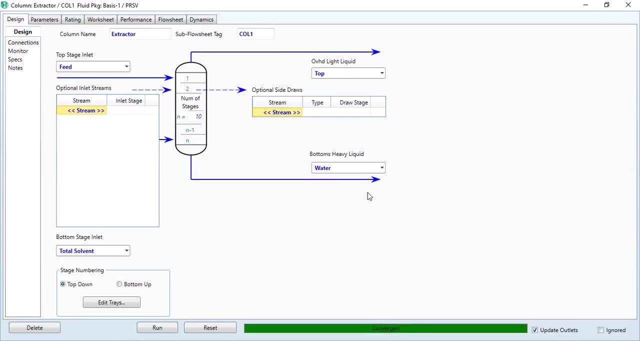 it as zero kg for R and in composition obviously it will be three methylhexane on mole basis. so it has converged successfully and the total solvent is placed over here now in bottom stage inlet, i will add total solvent and will run it and, as you see, this column has converged.